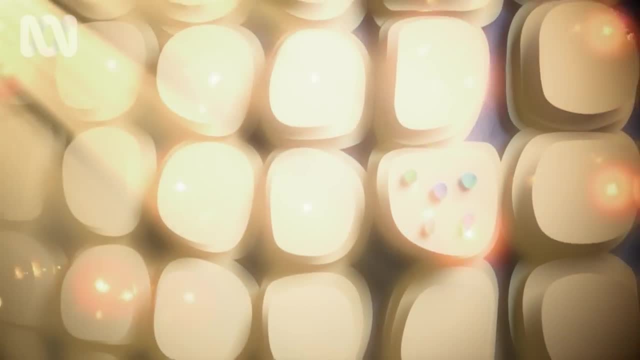 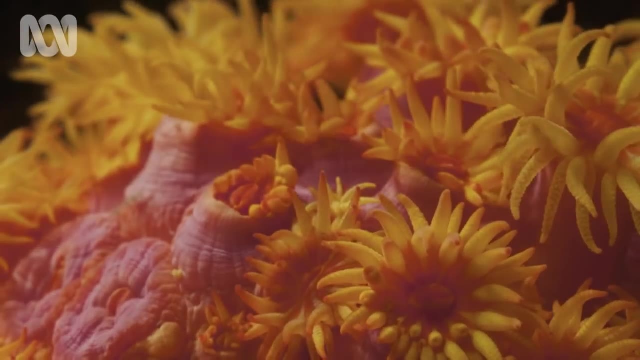 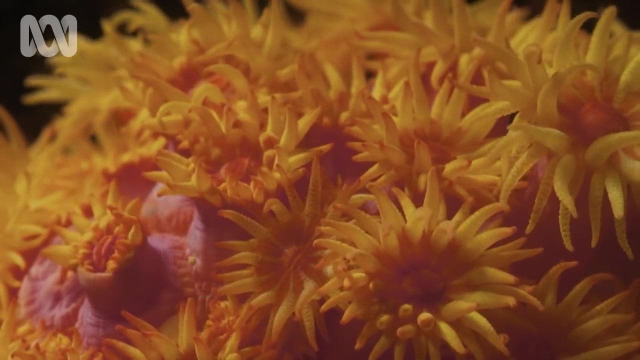 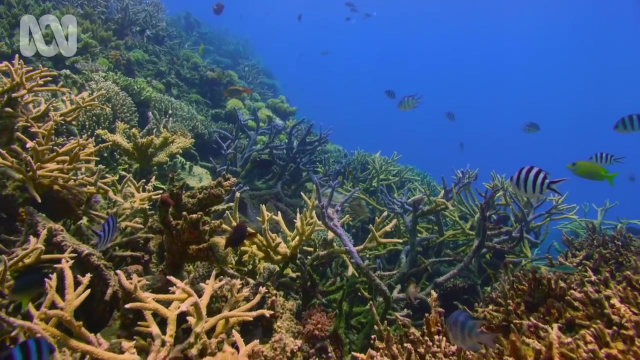 enough food for themselves and for their coral host. It's extraordinary biology, An almost alien relationship, where the algae gets a home and the coral gets up to 90% of its food, And together they build the reef. But because of warming oceans there's been a massive breakdown in this crucial relationship. 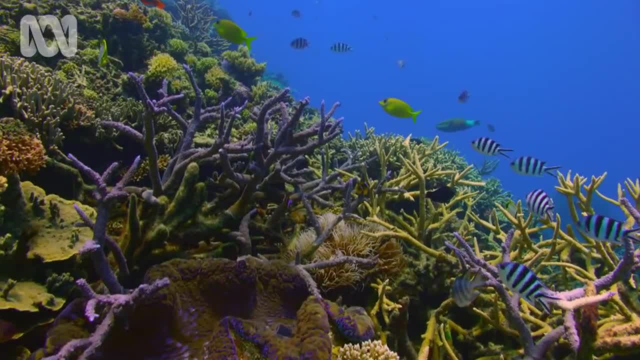 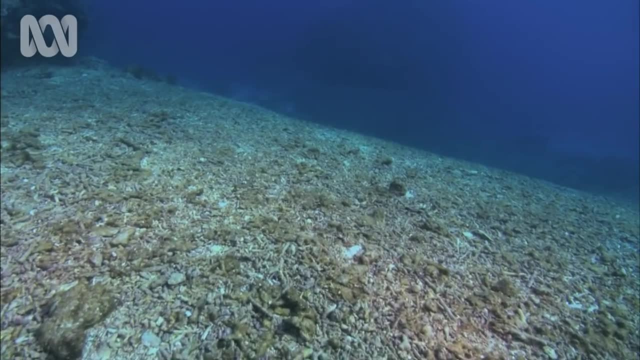 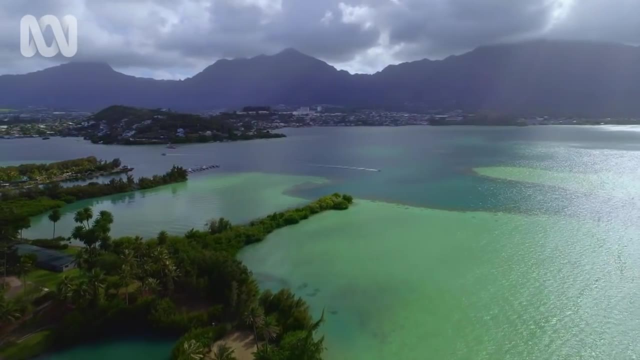 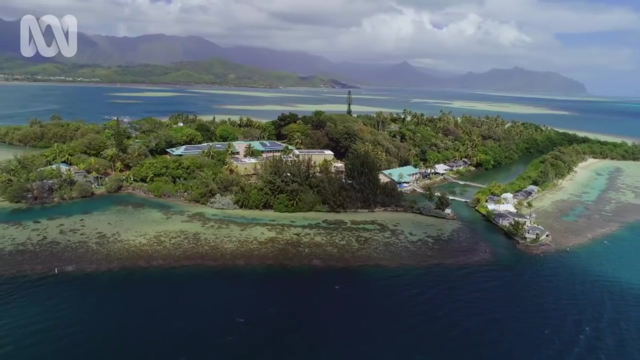 And the reef as we know it is disappearing. It's not just the coral that's disappearing, It's the coral that's growing faster. If science can help the reef survive, the answer may lay halfway around the world. On a tiny Hawaiian island, scientists are trying to understand the connection between coral and the plant inside them. 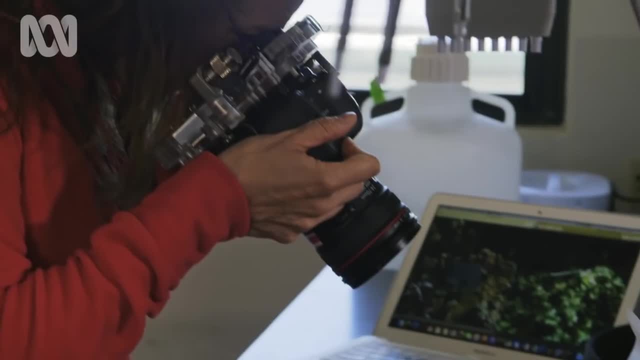 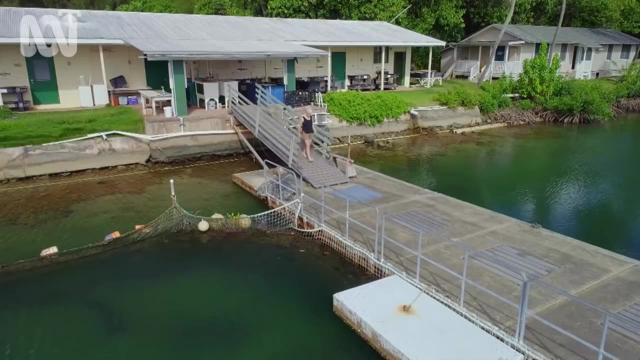 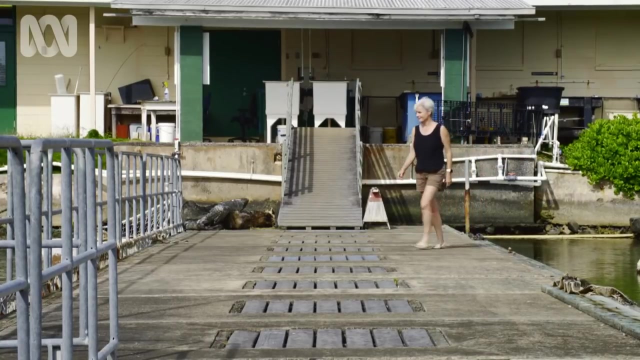 And use that knowledge to speed up evolution. And use that knowledge to speed up evolution. I'm at the Hawaiian Institute of Marine Biology where Ruth Gates does her research. It's an ideal facility. Over here you can grow corals And over here you can grow hammerhead sharks. 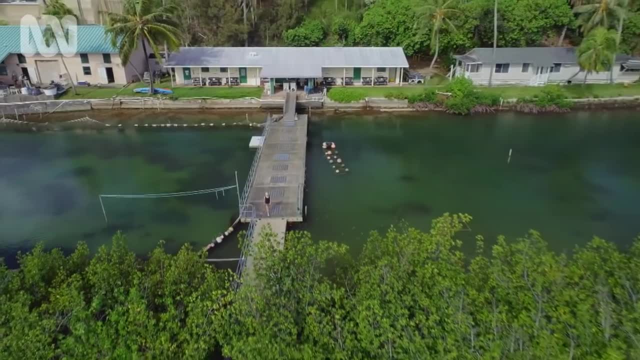 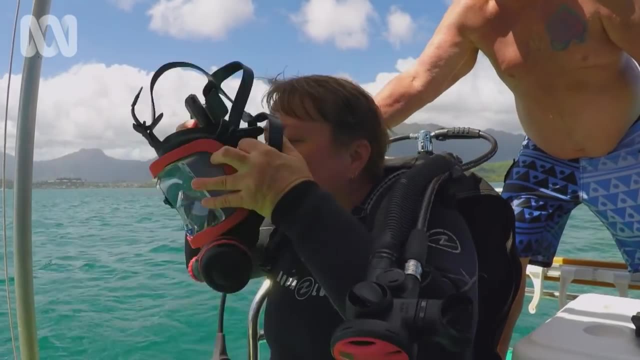 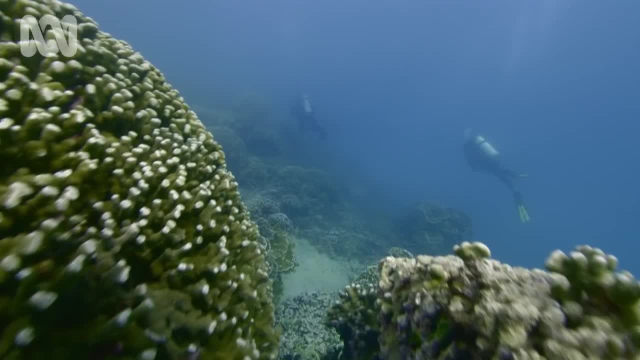 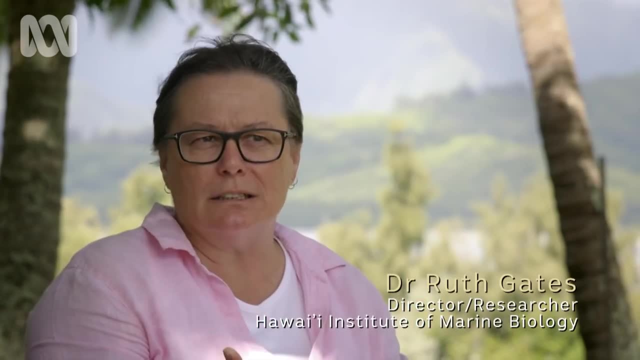 Dr Ruth Gates has been studying corals for over 20 years, Inspired by a love of the reef. The coral reef is a vibrant natural city. It's got texture, It's got colour, It's got movement. You're surrounded by extraordinary things. 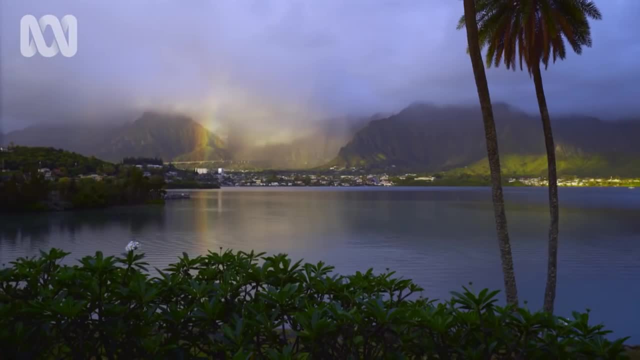 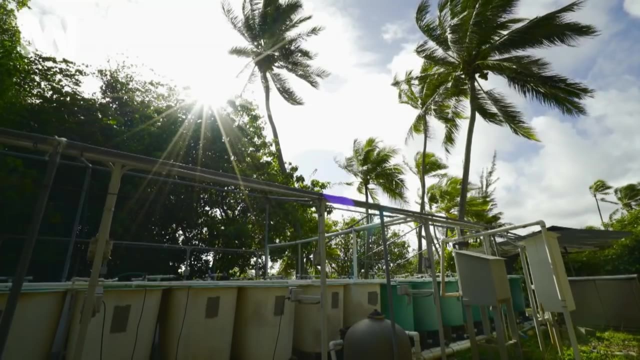 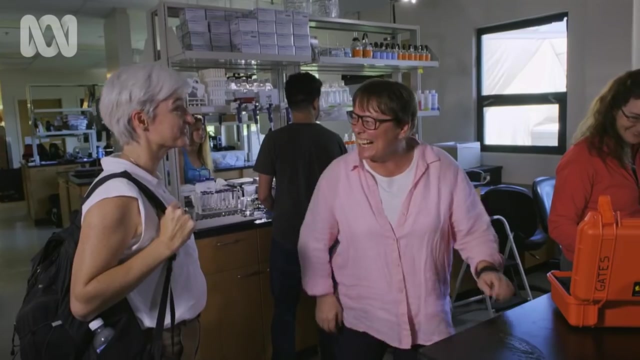 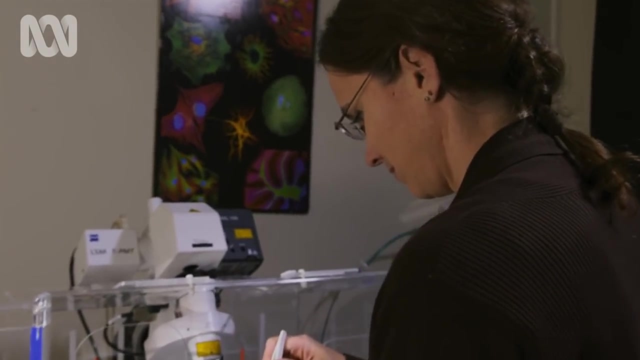 You're surrounded by extraordinary things. Ruth and her team are investigating the mechanism of coral bleaching. What happens when temperatures get too high for coral? What happens when temperatures get too high for coral? This special microscope lets Ruth and biologist Amy Eggers raise the water temperature to. 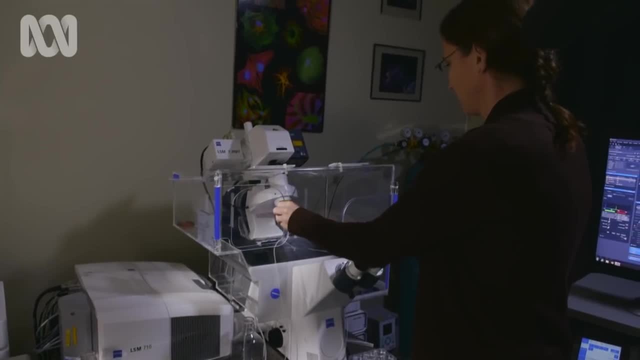 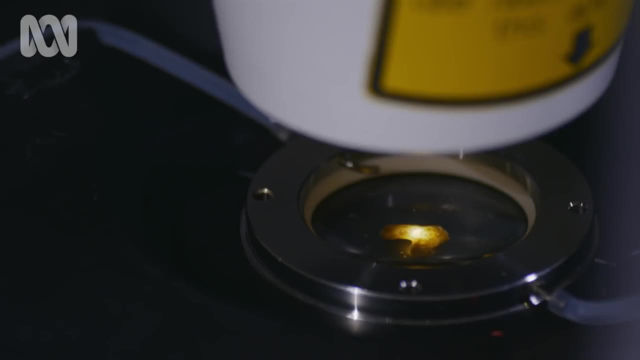 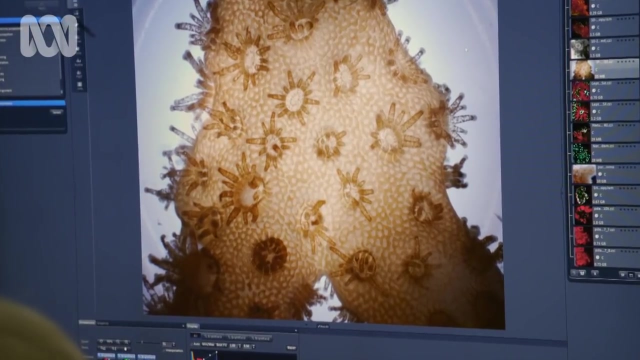 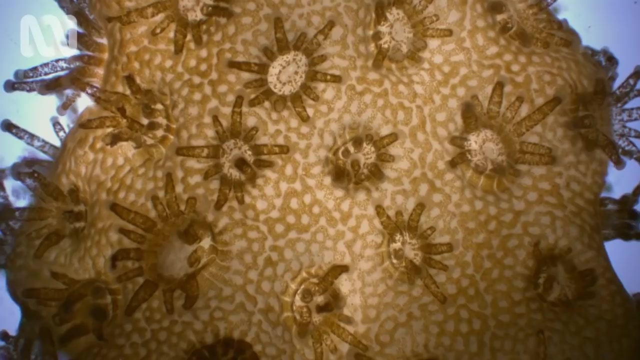 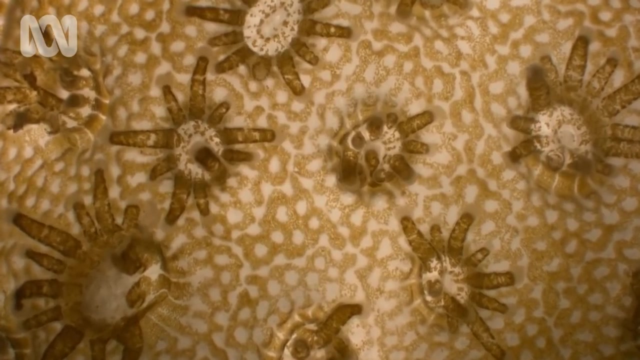 simulate warming oceans and observe what happens to living coral as it bleaches. This is the only microscope in the world that's equipped to simulate future ocean conditions. that allows you to visualise a living organism, So you can really see how it's a colonial animal here, can't you All of those polyps? 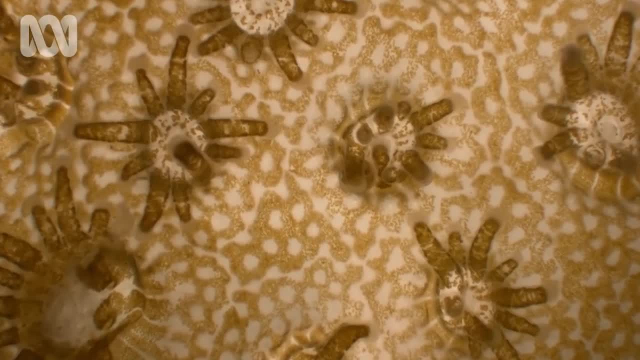 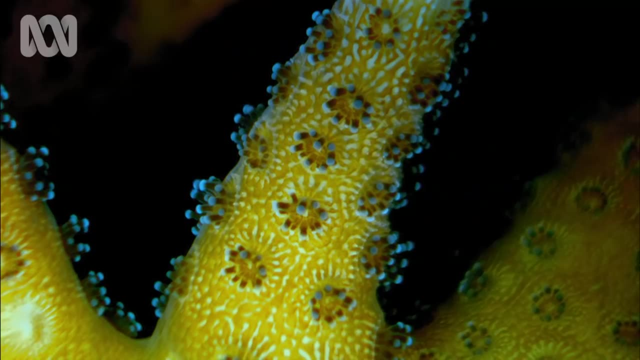 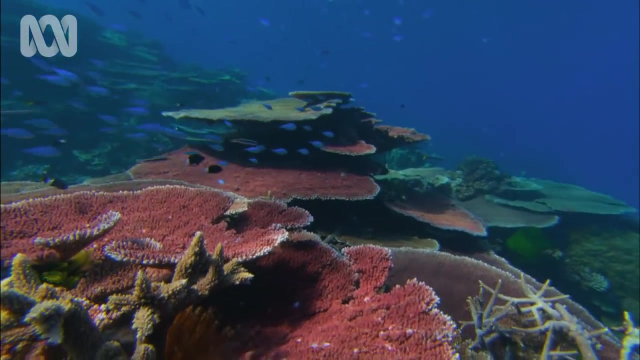 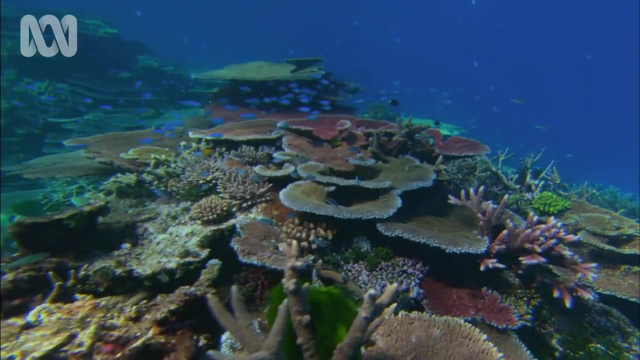 The number of algal cells, or symbionts, living throughout the coral is staggering: Around a million in every square centimetre, an area the size of your thumbnail. Coral builds the reef structure that supports so much other life, So it's called a foundation. 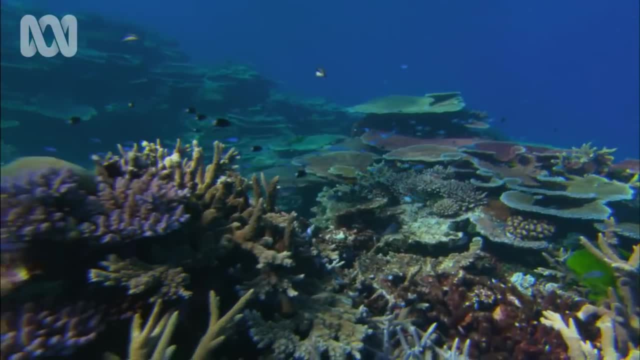 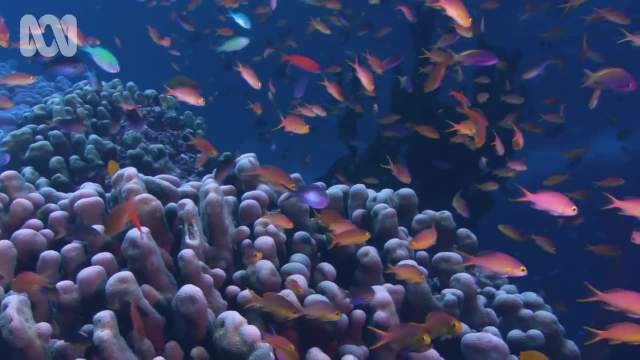 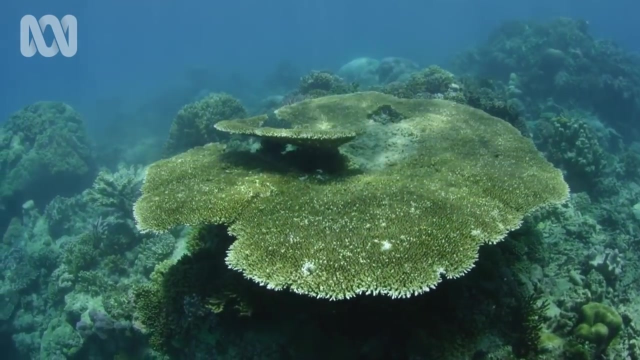 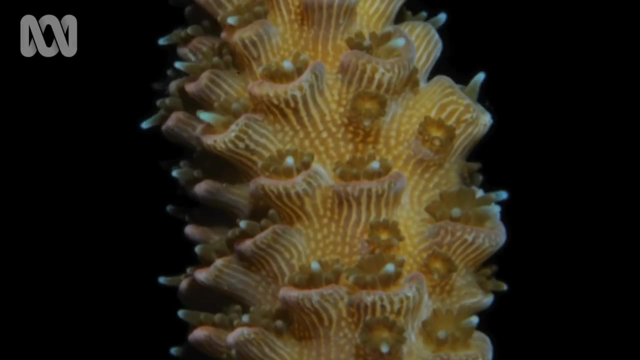 species. If coral is a foundation species, then the symbionts themselves are clearly a keystone species, because the coral cannot survive without them. And if the coral doesn't survive, the reef will not survive. Adam. When ocean temperatures get too high, the coral rejects the algae living inside it in. 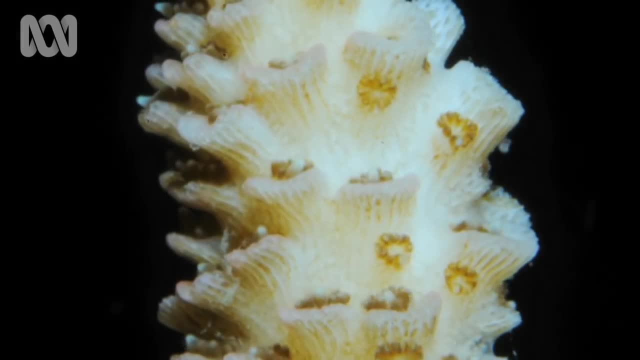 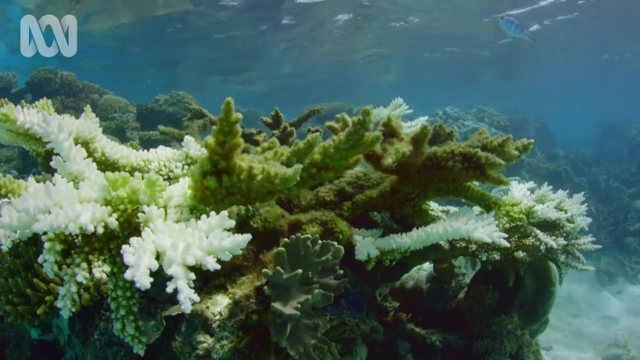 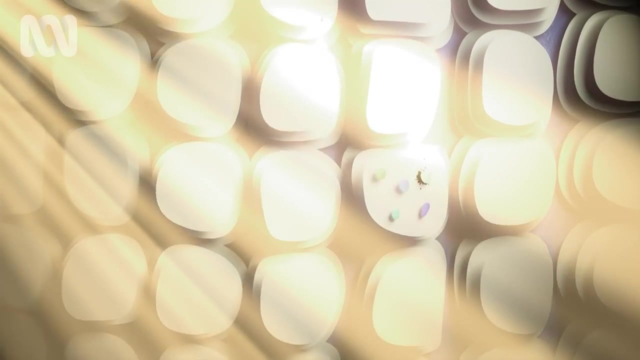 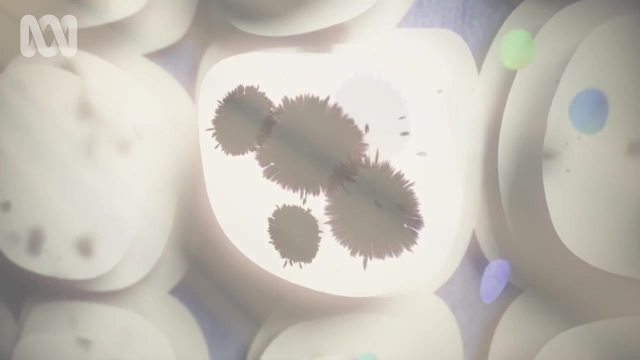 the process called bleaching Edwin Coral. bleaching is really the breakdown of this relationship between these plant cells and the animal itself. The plant cells react to high temperature to remove the Grow-2. when берu Coral Storm, creating food, they produce an irritant to the coral When the animal gets. 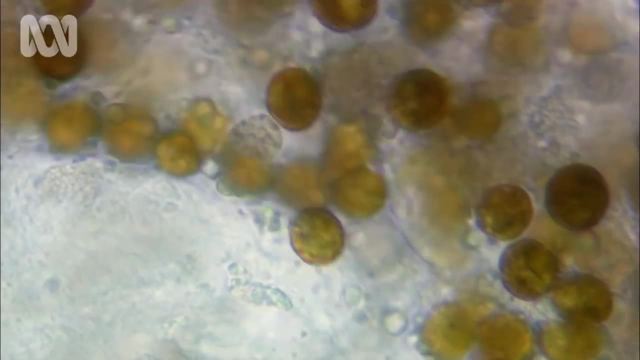 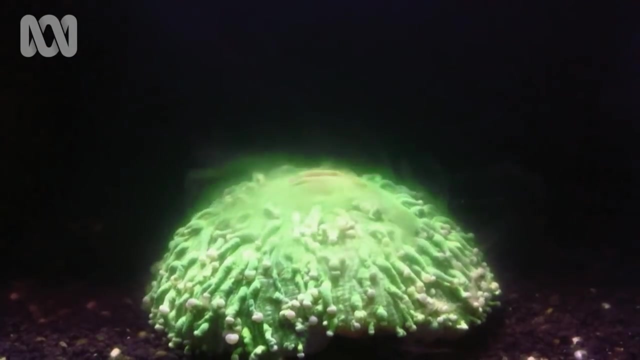 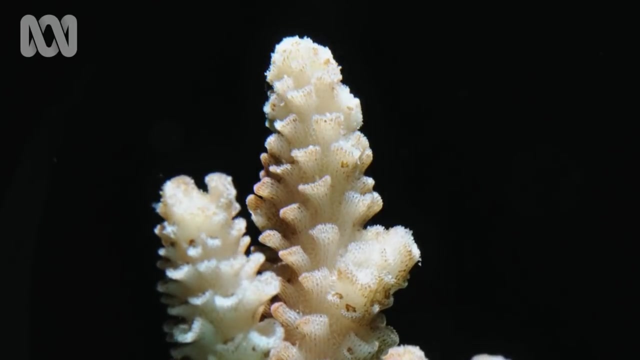 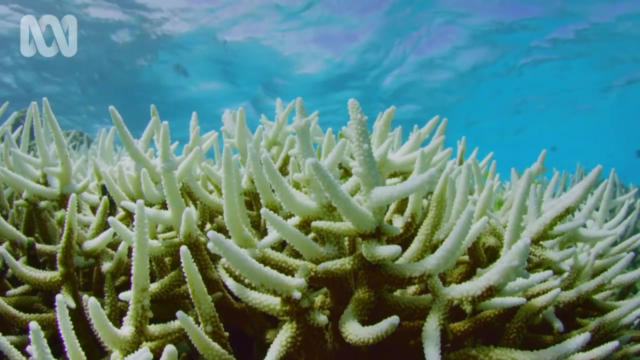 stressed. somehow they break the connection and the plant cells are ousted from the system. Some corals belch clouds of their life-giving algal cells. Others release them over days in tiny clumps. What you see as the coral goes pale is just the clear tissues of the animal overlaying the white skeleton. 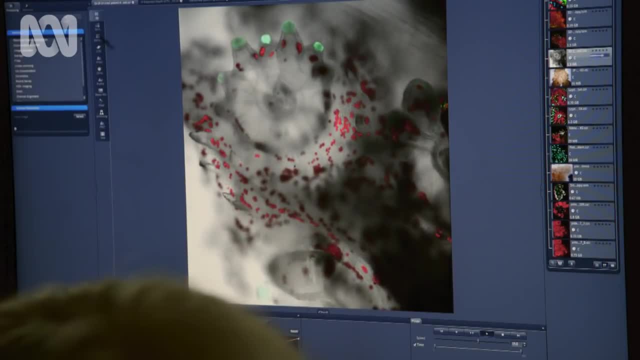 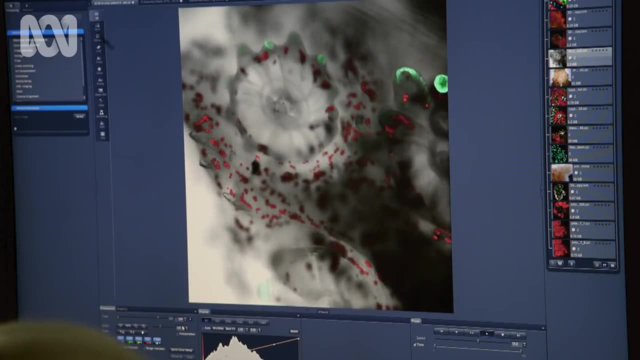 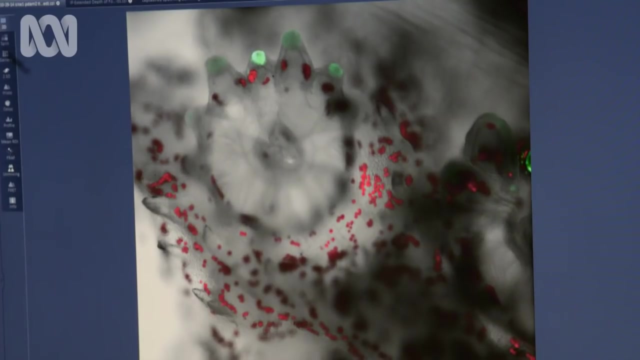 Bleached but still living coral can clearly be seen under powerful magnification. It's become a ghost coral, hasn't it Like? you know that all the structure is still there, but none of the colour, none of the vibrancy. That is a spooky image.